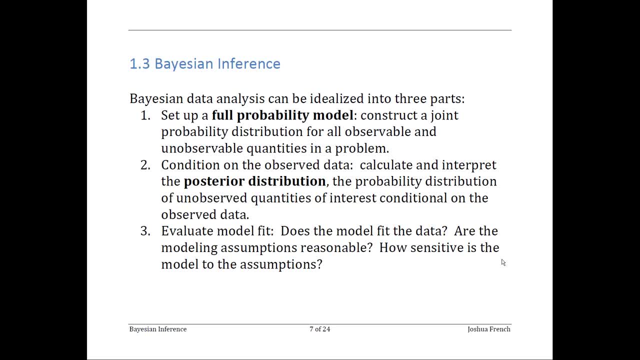 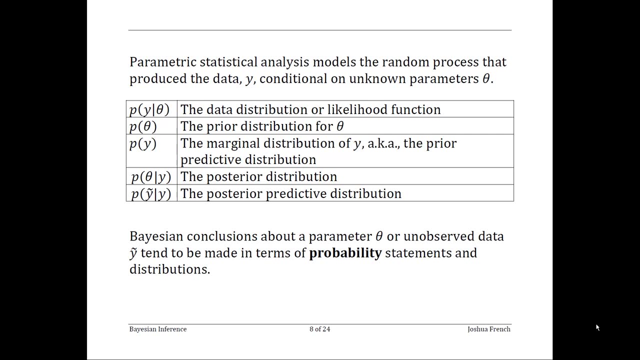 realistic or useful model to fit? How sensitive are your results to the probability model that you set up? Considering that third step, it may cause you to go back and change some of the initial steps and reiterate through the process. Let's talk a little bit more about the notation we're going to use to describe the various components. 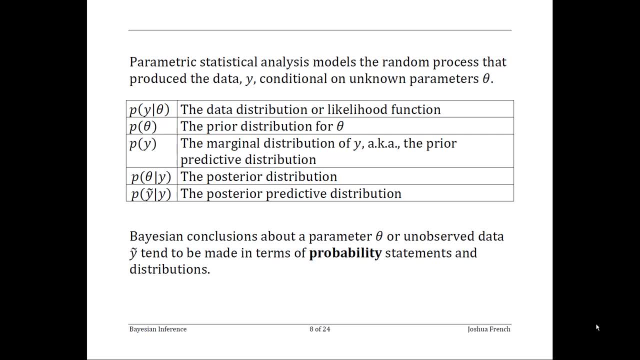 of our Bayesian model. A parametric statistical analysis models the random process that produces our data y conditional on some unknown parameters, which we are denoting by theta. In a Bayesian context, we're going to use very specific terms to describe the different distributions we're going to be working with. 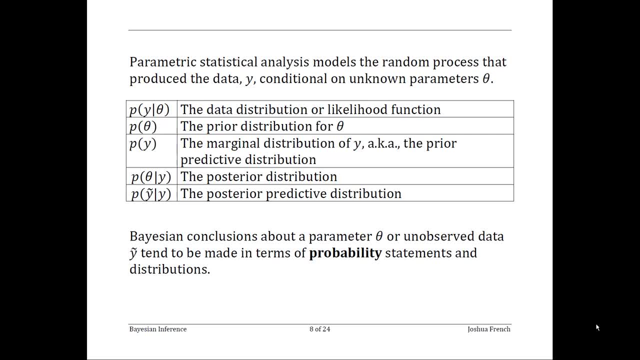 P is known as the data distribution or likelihood function. This is the model that we believe produced the data conditional on the model parameters and possibly some covariates. P is going to be used to denote the prior distribution about our vector of model parameters. P is going to denote: 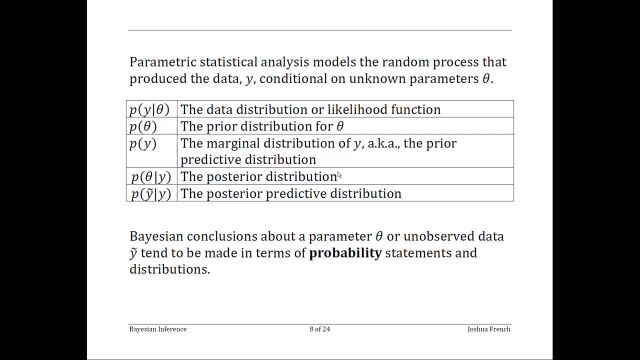 the marginal distribution of y. This is obtained by taking the joint distribution of y and theta and then, depending on whether the joint distribution is continuous or discrete, integrating or summing the joint distribution over the support of theta. The next distribution that we're going to talk about is very important, and that is P. 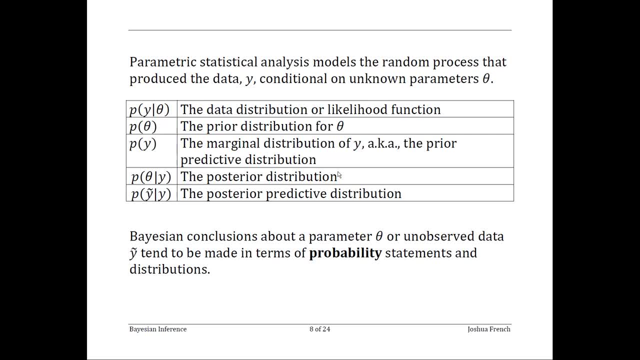 which is known as the posterior distribution. It's one of the main distributions that we seek in Bayesian statistics and that's closely followed by the posterior predictive distribution, P given y. We'll talk about both of these in a moment, But one of the things I want to point out is that both of these 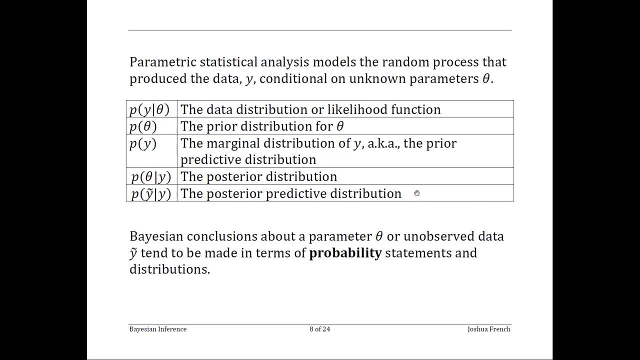 distributions that we're interested in learning about. in Bayesian statistics the posterior distribution and the posterior predictive distribution are in fact both distributions. In frequentist statistics we're usually after point estimates or point estimators and possibly the standard error associated with those things, But the quantities of interest in frequentist statistics are not. 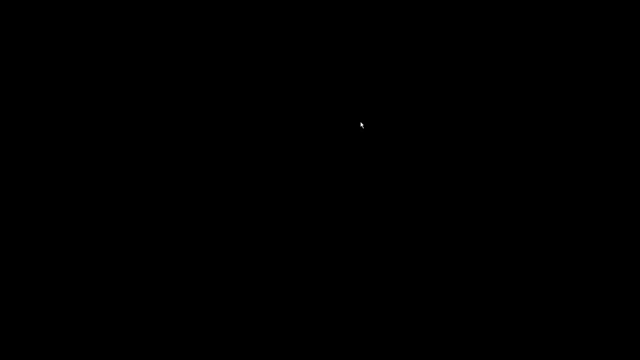 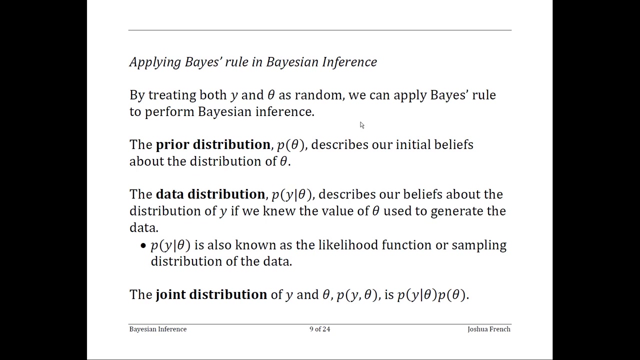 in fact distributions, whereas in Bayesian statistics they are. At this point you may be wondering exactly how we apply Bayes' rule in performing Bayesian inference, And the key ingredient is to treat both the observed data y and the parameter vector theta as being random. We have to give them. 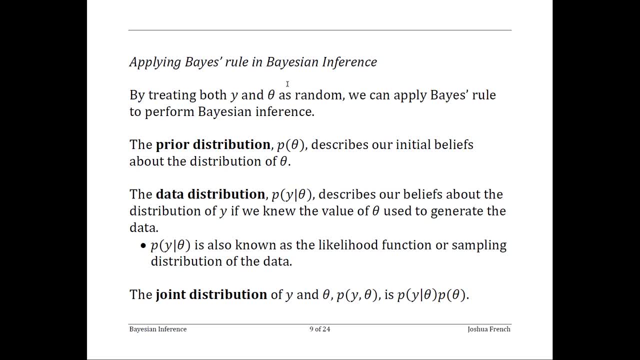 distributions. After doing that, we can apply Bayes' rule in performing Bayesian inference. The distribution of theta that we consider is the prior distribution, which describes our initial beliefs about the distribution of our parameter vector. This can be a very vague distribution if we don't know much about. 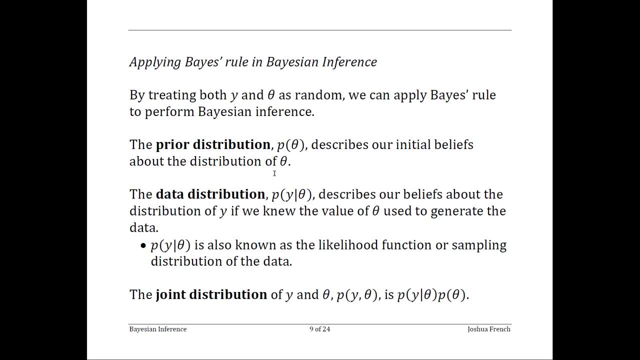 the parameter vector ahead of time, or it can be more compact or specific if we have some expert opinion to guide our beliefs. The data distribution is going to describe our beliefs about the process that generated the data. if, in fact, we knew what the parameter vector theta, actually was. 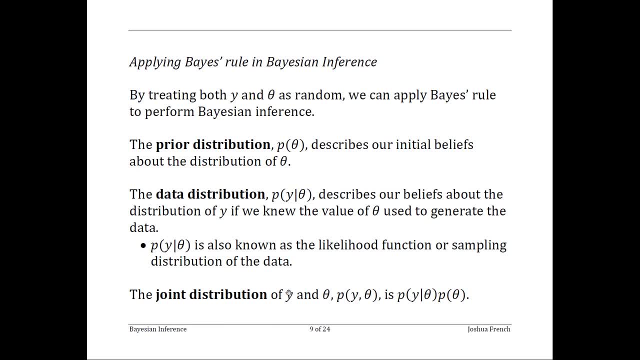 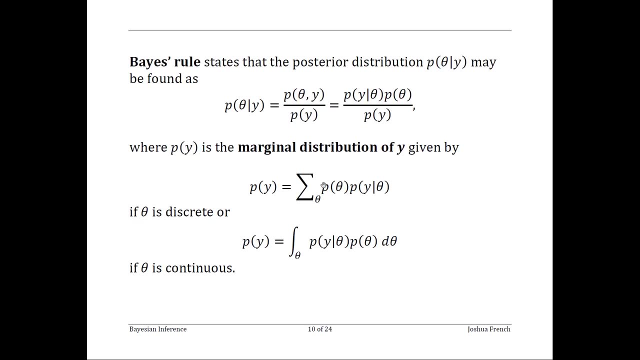 Using these two distributions allows us to construct the joint distribution of y and theta, p of y, given theta by taking the data distribution and multiplying it by the prior distribution. The last ingredient that we need is the marginal distribution of y, which is obtained by taking the joint distribution of y and theta, and. 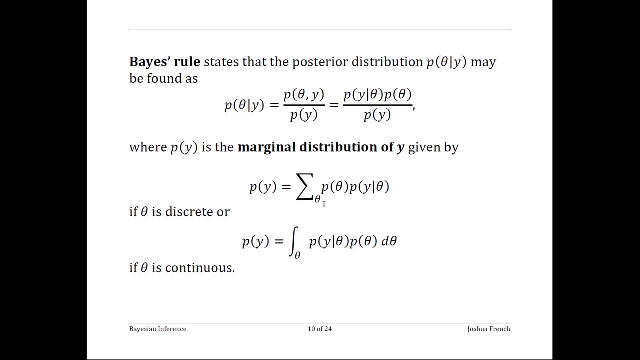 either summing over the values of theta, if that's a discrete distribution, or integrating over theta, if the theta parameter is a continuous random variable. Once we have the data distribution, the prior distribution for theta and the marginal distribution of y, we can obtain the posterior distribution p of theta. 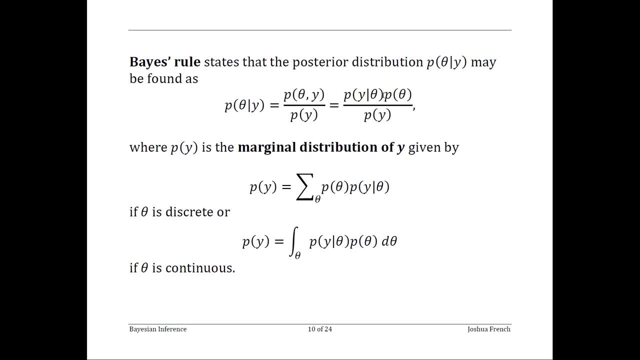 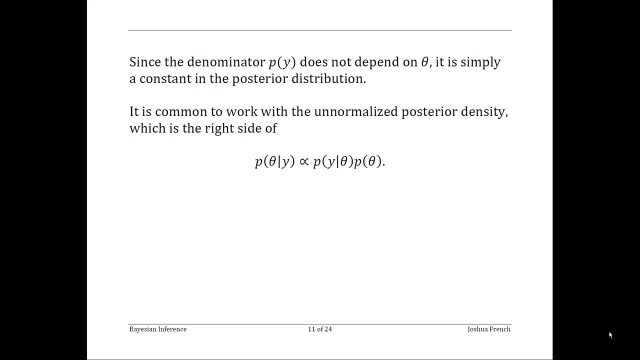 given y by taking the product of the data distribution and the prior distribution and dividing by the marginal distribution of y. One of the things to note in the previous formula for the posterior distribution on the last slide is that the marginal distribution of y in the denominator is actually a constant, because it's actually 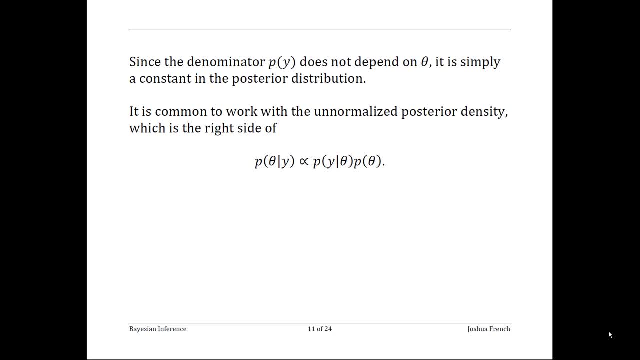 the distribution of the data evaluated at the observed values of y. Since it's a constant, we can usually ignore it when we're deriving our posterior distribution, since we know that the posterior distribution has to integrate to 1.. Thus, it's common to simply say that the posterior distribution is 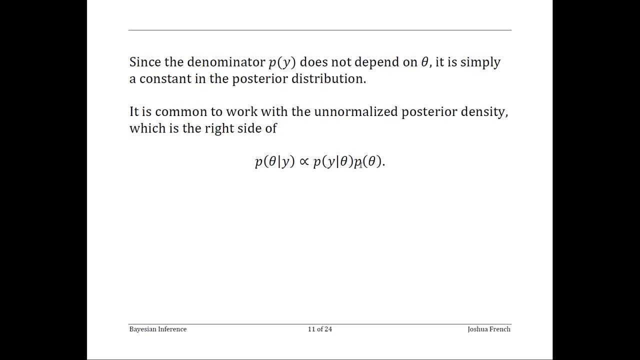 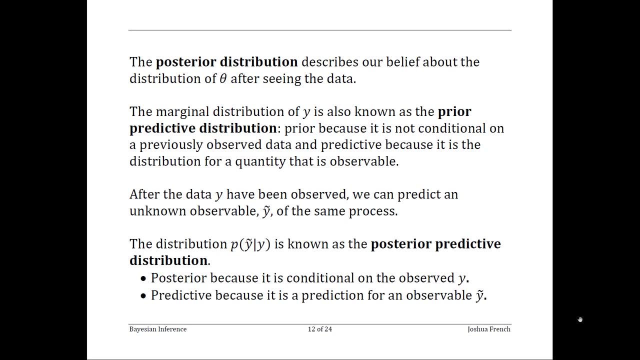 proportional to the data distribution multiplied by the prior distribution and ignore the scaling constant related to the marginal distribution of y evaluated at the observed data points. Let's talk a little bit more about the various distributions. we're interested in deriving The posterior distribution. what does it actually represent? Well, it describes. 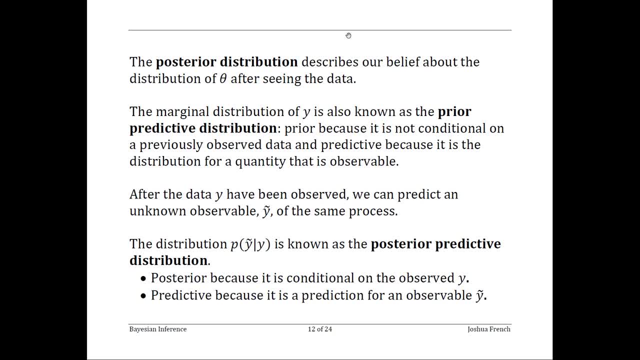 mathematically our updated beliefs about the distribution of our parameter vector theta. after seeing the data, We initially start with some beliefs described by our prior distribution, but then, after seeing the data, we update our beliefs, which is represented by the posterior distribution. 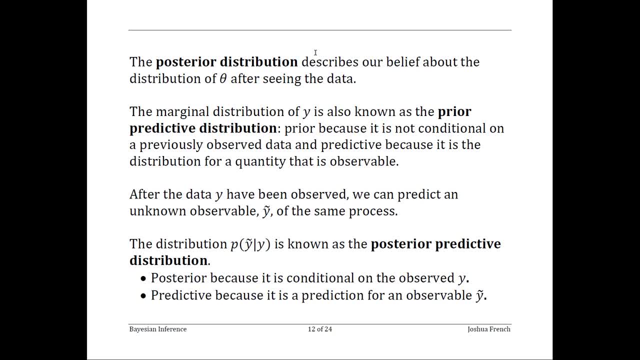 The marginal distribution of y is sometimes known as the prior predictive distribution. The word prior is thrown in because it's not conditional on observed data and it's a predictive distribution because it is a distribution for a quantity that is observable. The posterior predictive distribution p given y, is our beliefs. 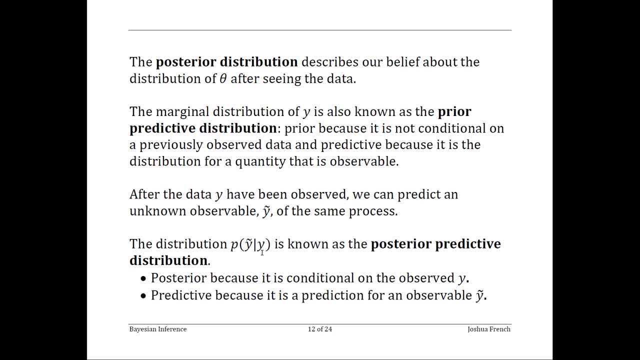 about the observable quantity y tilde after observing the data. Note that this distribution automatically accounts for any uncertainty in our parameter vector theta, the unobservable model parameters. It's called the posterior because it is conditional on the observed data and it's also called predictive because it is a distribution for an. 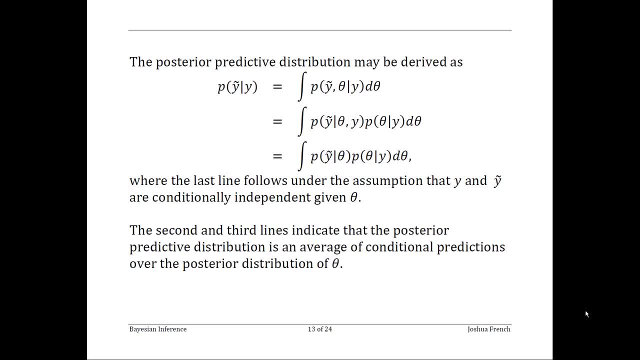 observable quantity. The posterior predictive distribution can be a pretty mystifying quantity when you first start Bayesian statistics. so I have a set of inequalities here. to try to demystify it to some extent On line 1, starting with the notation for the posterior. 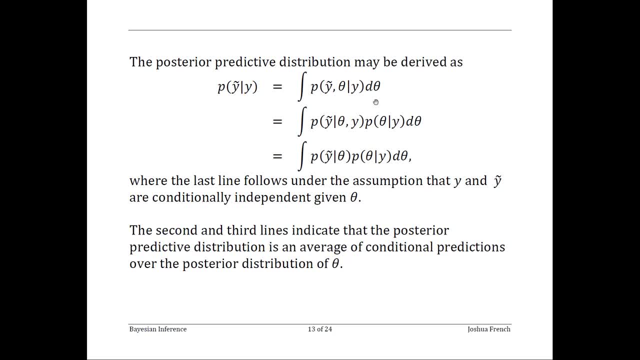 predictive distribution, we reverse the process of integrating theta out of the joint posterior distribution of y, tilde and theta. On line 2, we use the properties about conditional distributions to rewrite the joint posterior distribution of y, tilde and theta as the product of the conditional distribution of y- tilde- conditioned. 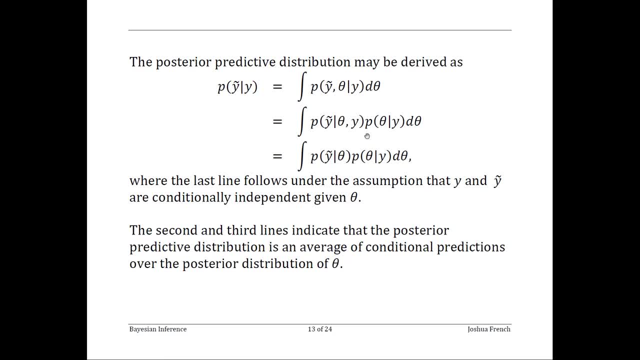 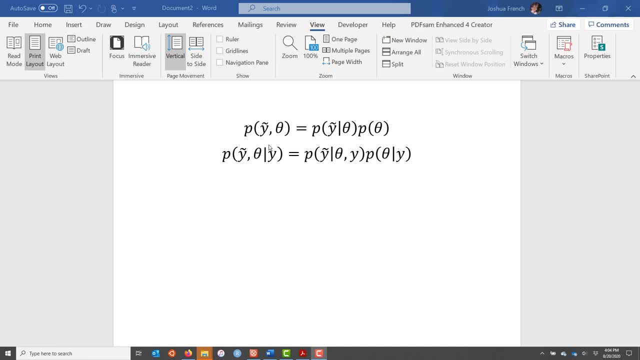 on theta and y multiplied by the posterior distribution of theta. That last step may seem a bit mysterious. If that's the case, just imagine writing the joint distribution of y tilde and theta as the product of the conditional distribution of y tilde, given theta multiplied by the prior. 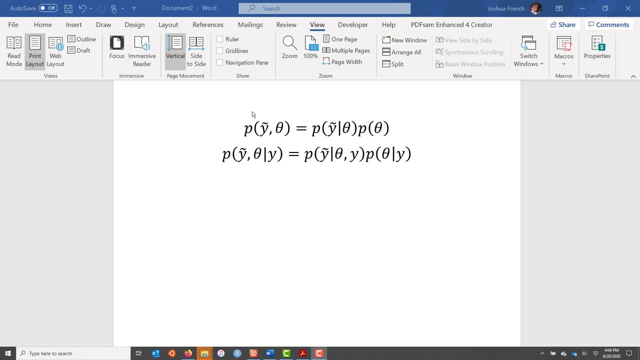 distribution p of theta. This follows pretty straightforwardly from the typical rules about conditional distributions. The fact that we're conditioning on the observed data y in each of these statements doesn't change any of the usual probability rules, and so I can take all of these. 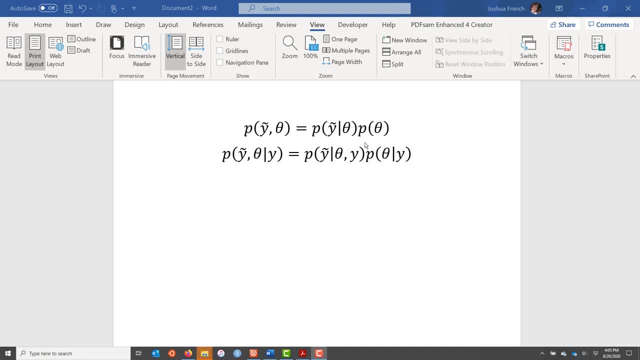 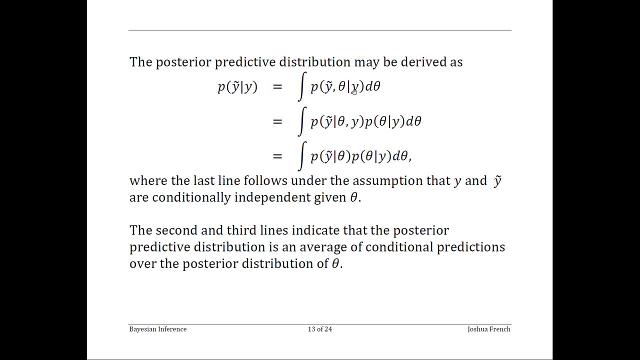 probability distributions, condition, each one of them on y, and the probability equality would still hold. Now let's get back to our set of equalities here. If we move between the second and third lines, we see that the only thing that we've done here is drop the dependence of this distribution.